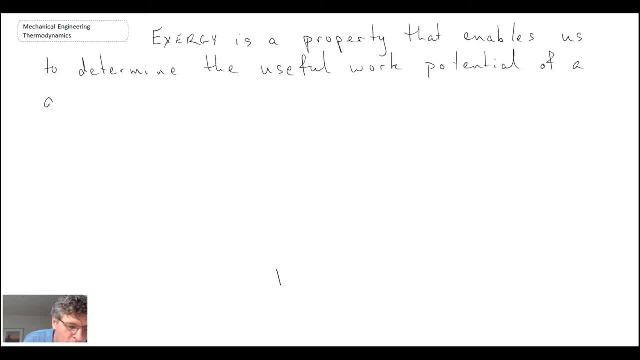 So what I'd like to do now is take a few moments to introduce the idea of exergy. So what I'd like to do now is take a few moments to introduce the idea of exergy. So what I'd like to do now is take a few moments to introduce the idea of exergy. 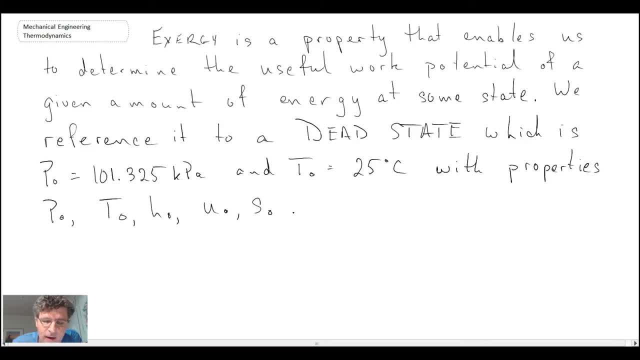 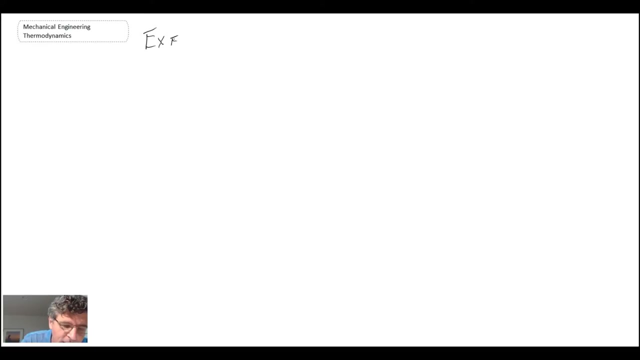